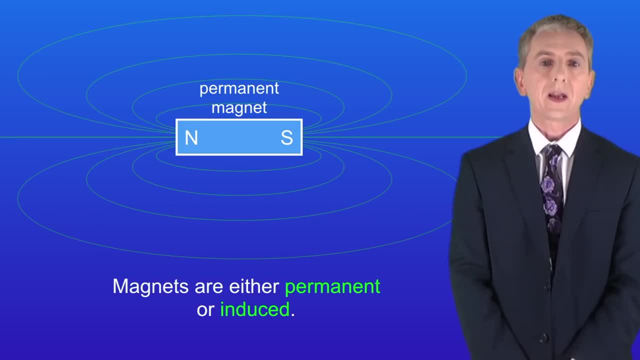 the evidence that the Earth's core is magnetic. In the last video we saw that magnets are either permanent or induced. A permanent magnet always has a magnetic field and I'm showing you here the magnetic field around a bar magnet. An induced magnet is a material. 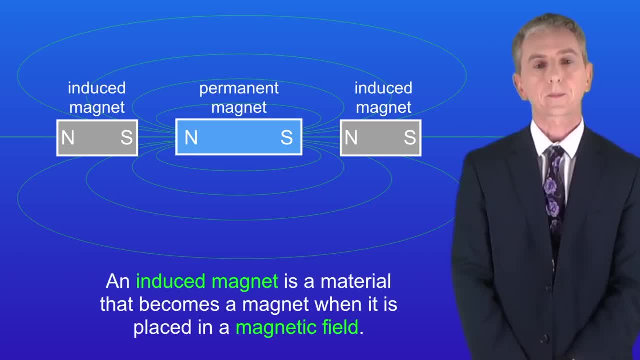 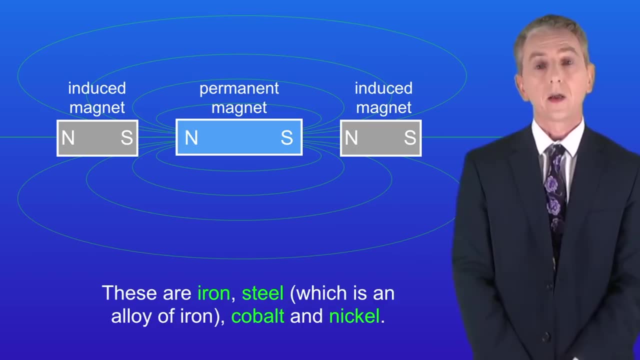 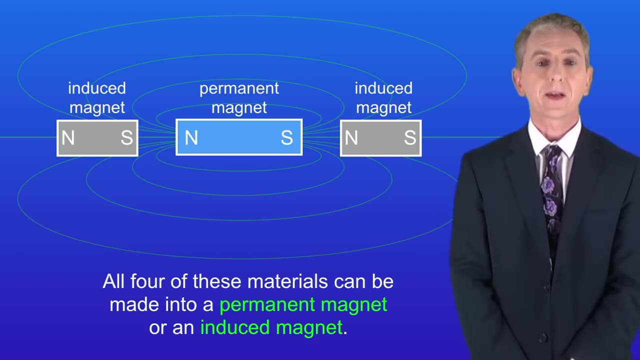 that becomes a magnet when it's placed in a magnetic field. Now, a key fact that you have to learn is that there are four types of magnetic material. These are iron, steel, which is an alloy of iron, cobalt and nickel. All four of these materials can be made into. 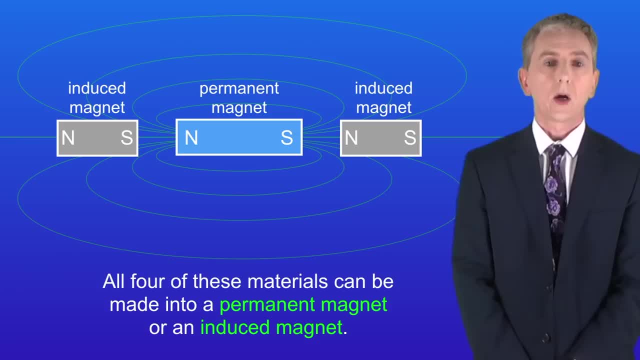 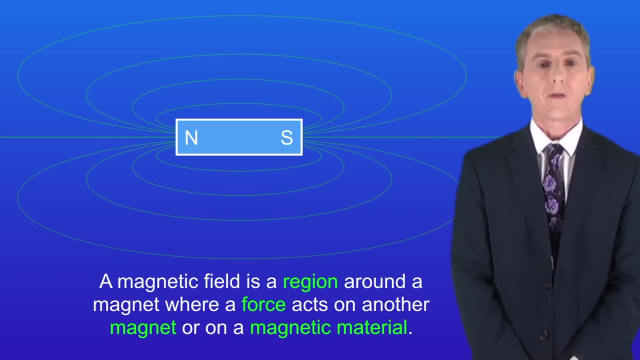 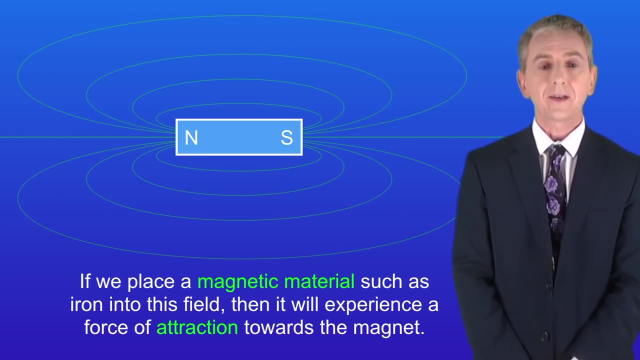 a permanent magnet or an induced magnet. Okay, so in this video we're looking at magnetic fields. A magnetic field is a region around a magnet where a force acts on another magnet or on a magnetic material. If we place a magnetic material such as iron into this field, then it will experience a force of attraction towards. 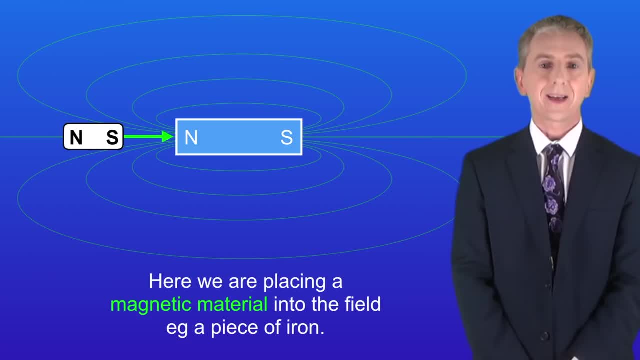 the magnet. So here we're placing a magnetic material into the field. for example, a piece of iron now becomes an induced magnet. This is now attracted to the permanent magnet. Now the strength of the magnetic field depends on the distance from the magnet. So here's. 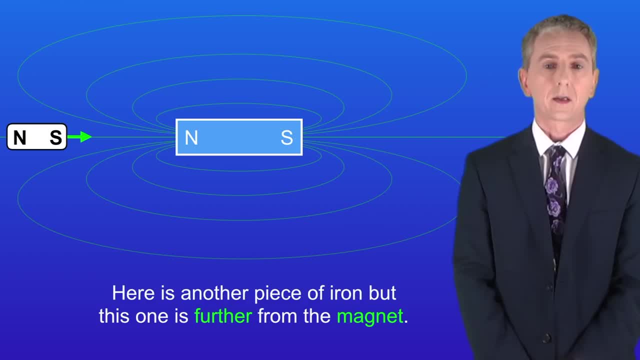 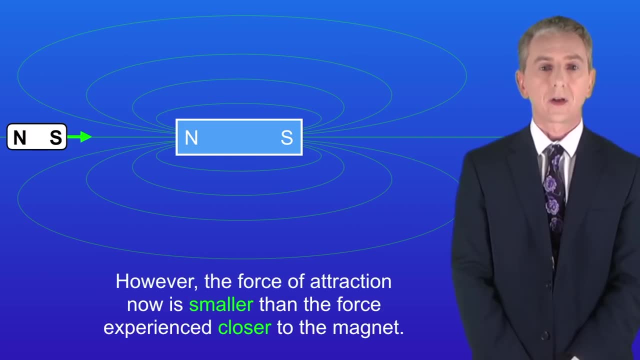 another piece of iron, but this one is further from the magnet. As you can see, the iron still experiences a force of attraction towards the magnet. However, the force of attraction now is smaller than the force experienced closer to the magnet. The field is also strongest. 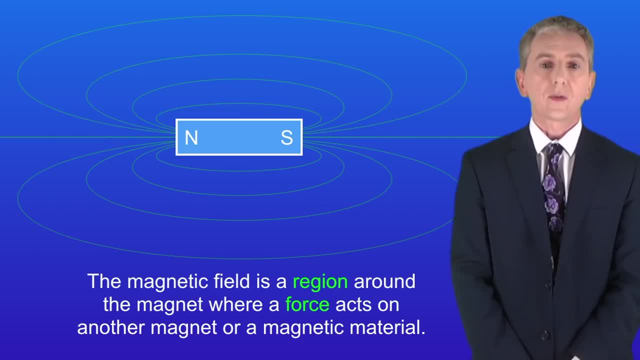 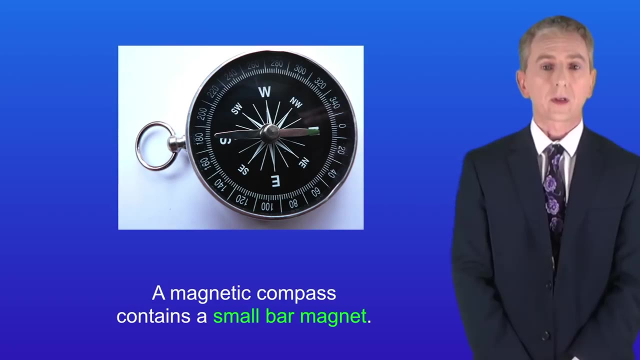 at the poles of the magnet. Okay, so, as we've said, the magnetic field is a region around the magnet, where a force acts on another magnet or a magnetic material. Now, the direction of a magnetic field can be found using a compass. A magnetic compass such as this one contains a small bar magnet. 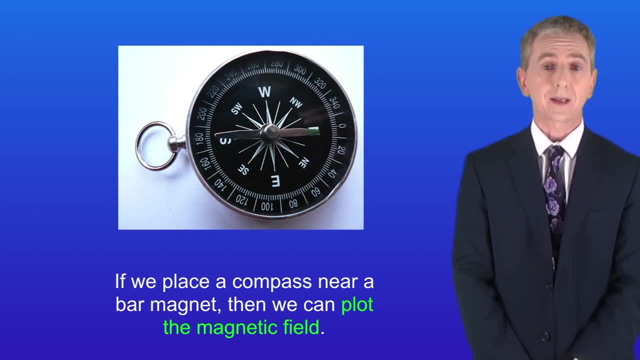 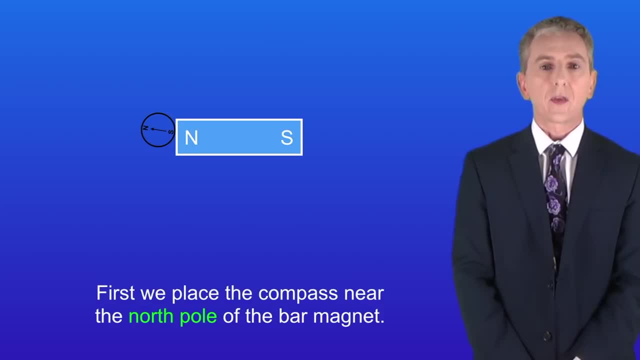 If we place a compass near a bar magnet then we can plot the magnetic field. So I'm showing you here the bar magnet and the compass. First we place the compass near the north pole of the bar magnet. We then draw a cross at the north pole of the compass. like this We now: 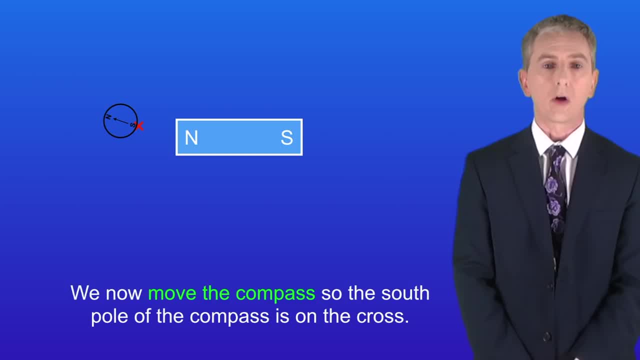 move the compass, so the south pole of the compass is on the cross, And again we draw another cross at the north pole of the compass. We continue doing this until we've plotted a complete magnetic field line. Now we connect all the dots with a line like this And we 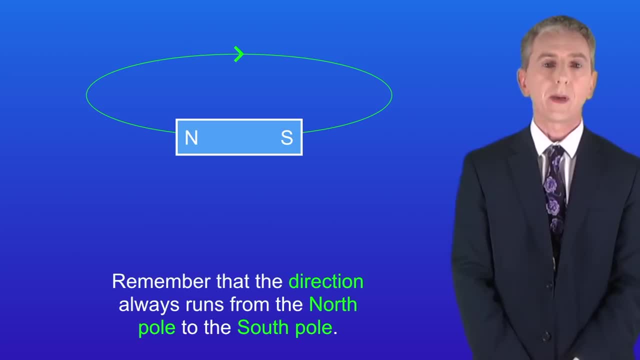 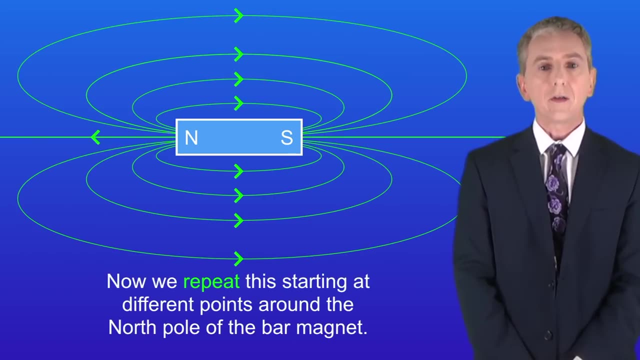 show the direction of the field line by using an arrow. Remember that the direction always comes from the north pole to the south pole. Now we repeat this, starting at different points around the north pole of the bar magnet. So this shows the magnetic field around a bar. 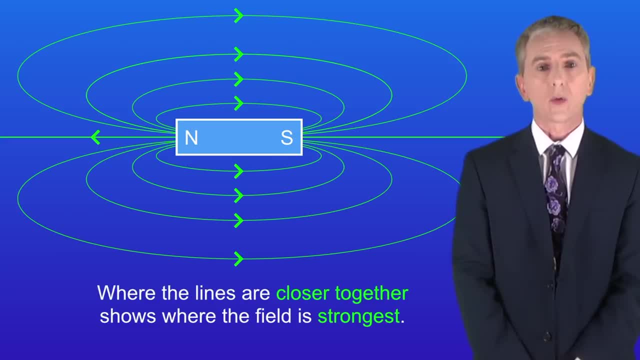 magnet, Where the lines are closer together, shows where the magnetic field is strongest. And, as we said before, the strongest part of the field is at the poles of the magnet. Okay, we're going to finish now by looking at the Earth's magnetic field We saw earlier. 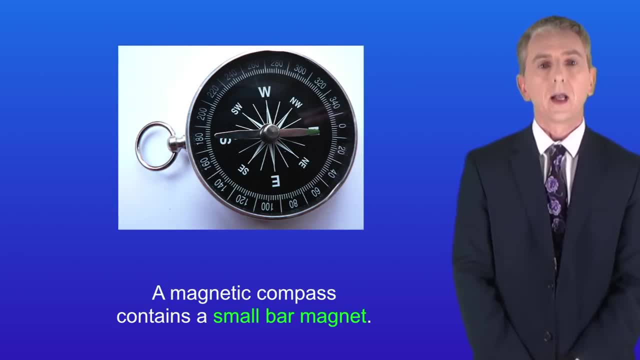 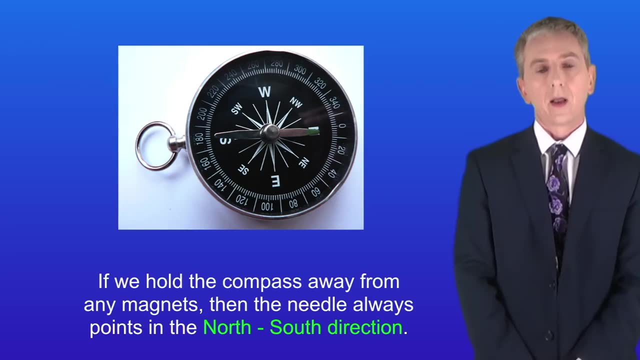 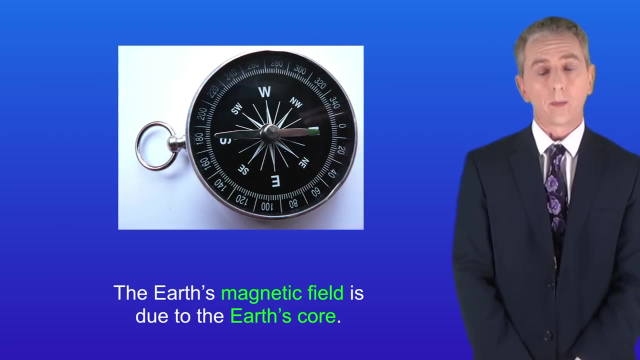 that a magnetic compass contains a small bar magnet. If we hold the compass away from any magnets, then the needle always points in the north- south direction. This tells us that the Earth has its own magnetic field And the Earth's magnetic field is due to the Earth's core. Remember. you'll find plenty of questions on. 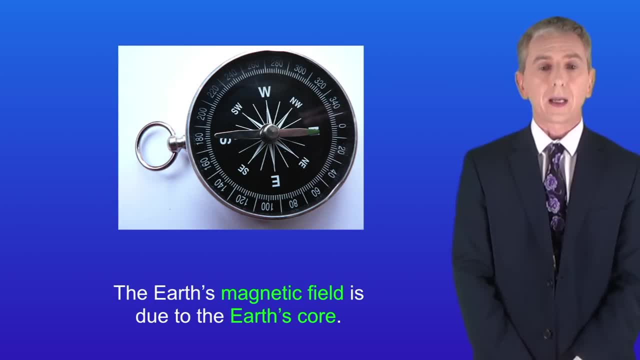 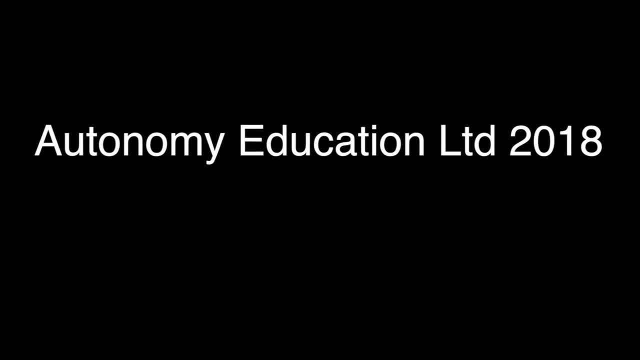 magnetic fields in my vision workbook And you can get that by clicking on the link above. Thank you for watching and I'll see you in the next video. 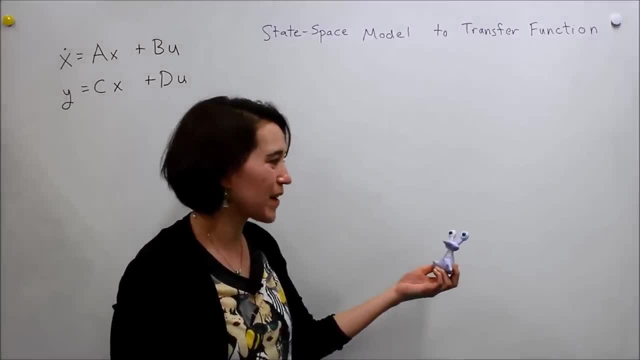 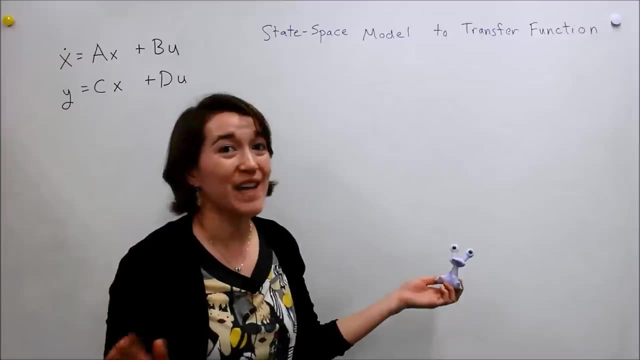 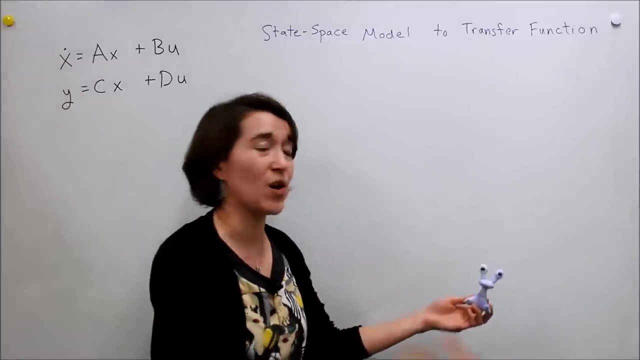 You like the transfer functions better than state-space modeling? Oh, I can't believe it. Well, it's not better, It's different. Well, if you like transfer functions, or want to use the transfer function rather than state-space, or you want to model in state-space and then go to the transfer function,